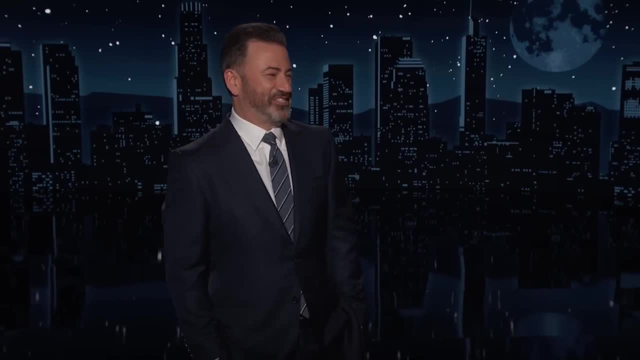 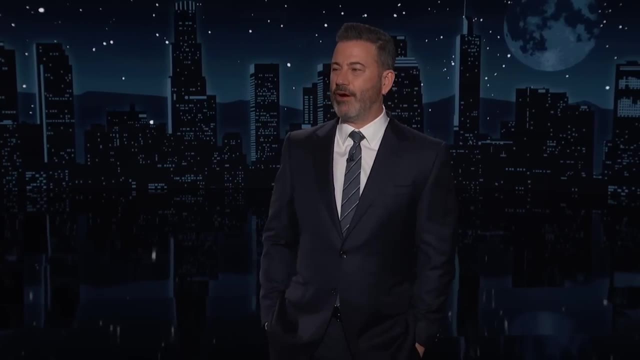 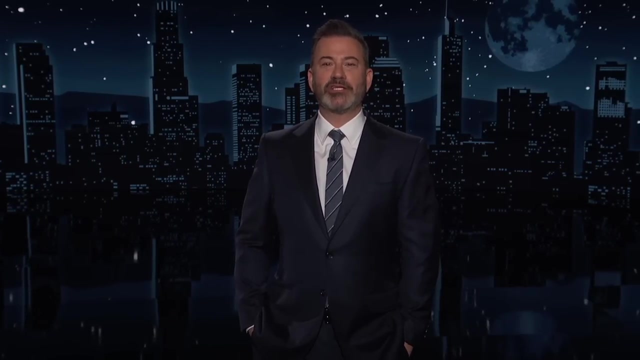 That's right. Don't don't be silly. There's just no time for malarkey and we won't tolerate it If Biden wasn't alone. you can tell how little faith our doctors, our scientists, even our news organizations have in us by the amount of times they had to tell us. 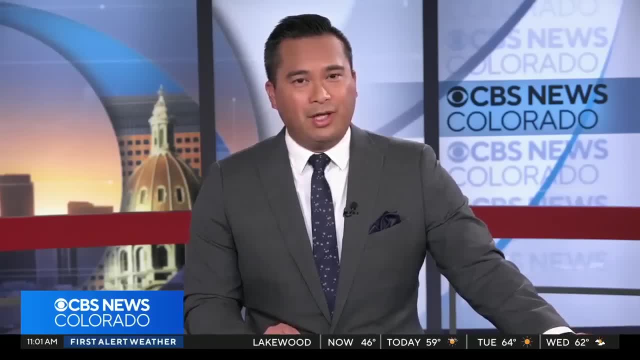 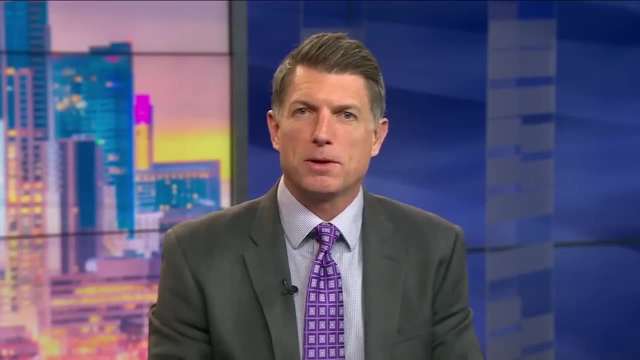 not to look directly at the sun today. Today is the solar eclipse And a reminder, if you still haven't heard: do not look directly at the sun without proper glasses. Eye doctors are warning people. Do not look at the sun. I have to tell you. don't look at the sun. 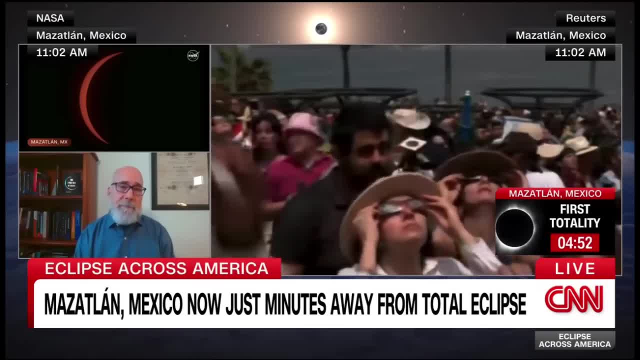 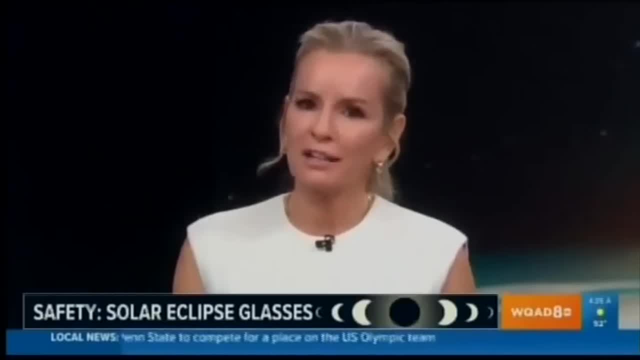 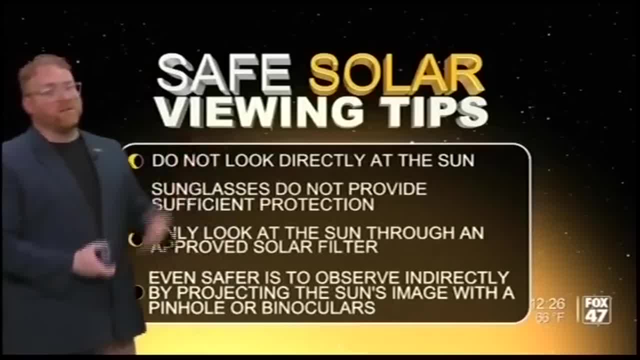 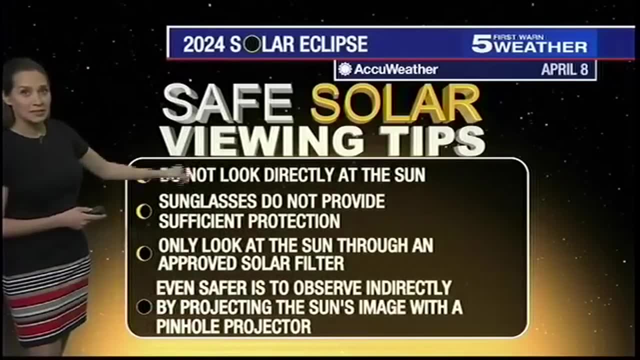 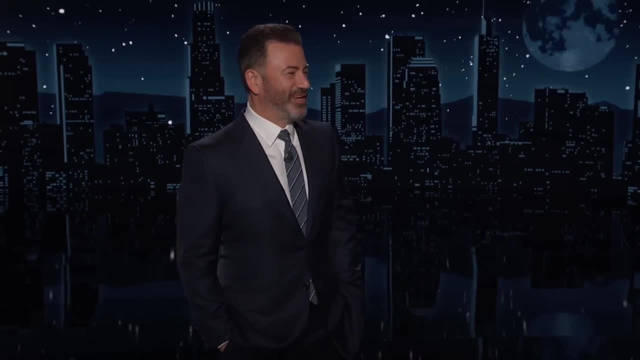 Yeah, that's easy, And yet somehow we have to look directly at the sun. And yet somehow we have to look directly at the sun. And yet somehow we have to look directly at the sun, And yet somehow it makes me want to look directly at the son. 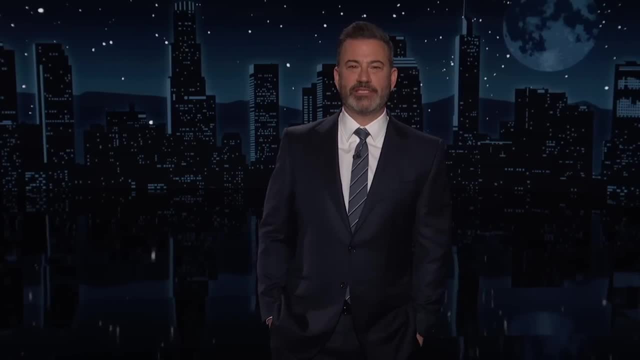 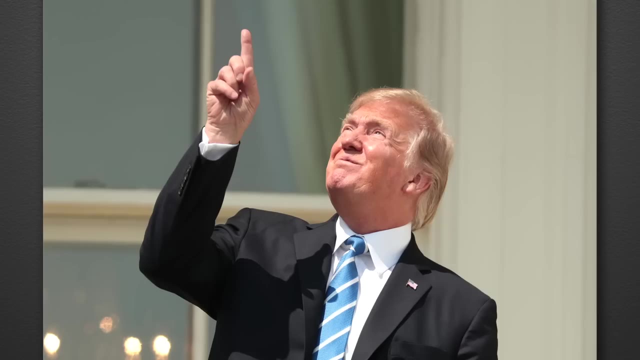 You know, the last time the son dared to pull a stunt like this was in 2017, when our then leader stared directly at it And he said: not today, son, Not today He wasn't wearing any wimpy cardboard glasses. 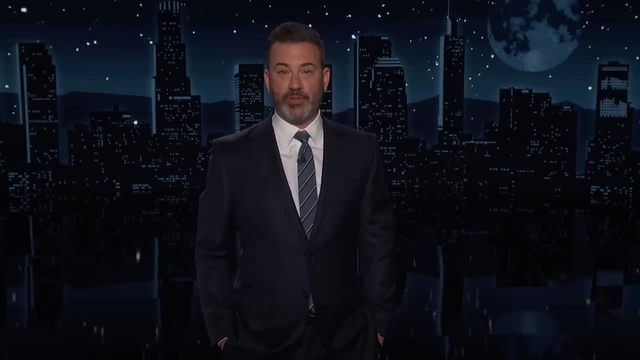 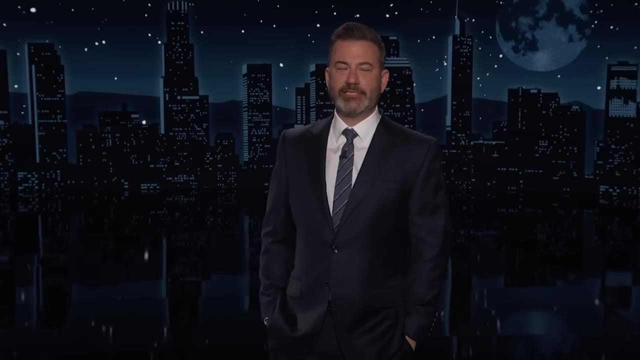 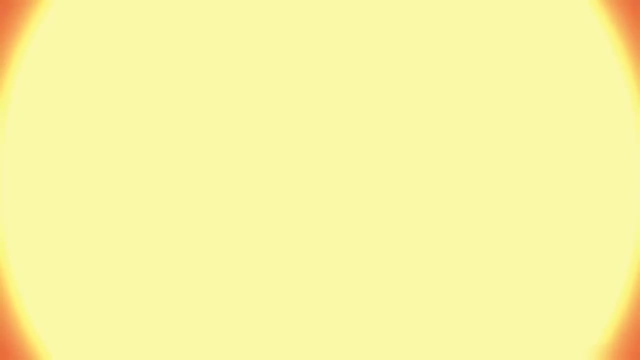 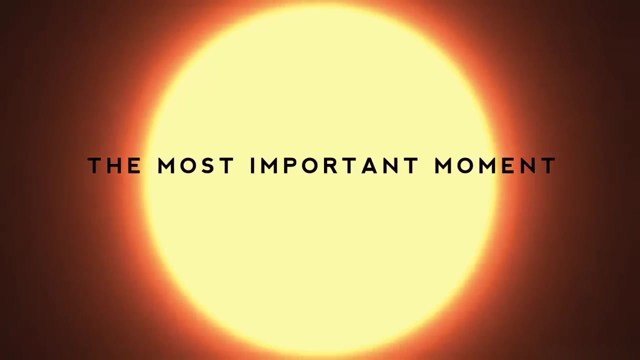 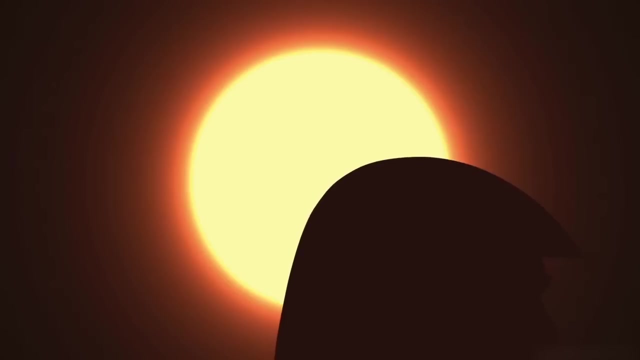 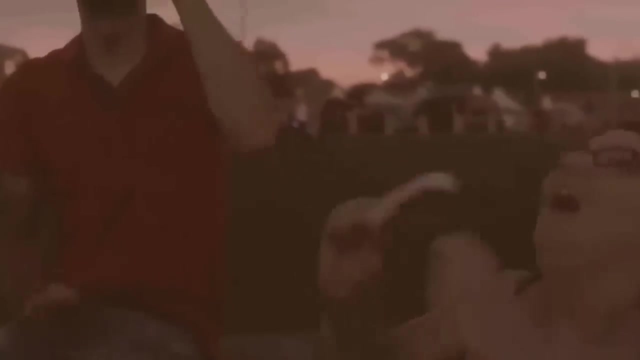 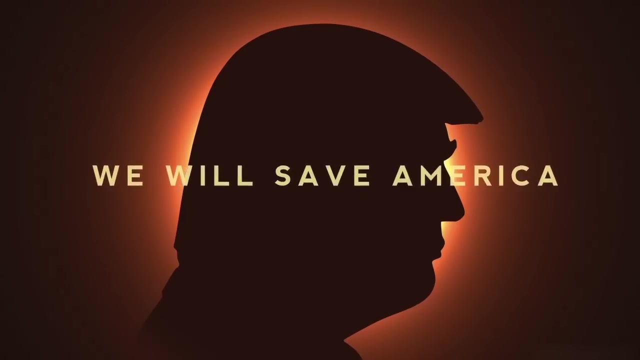 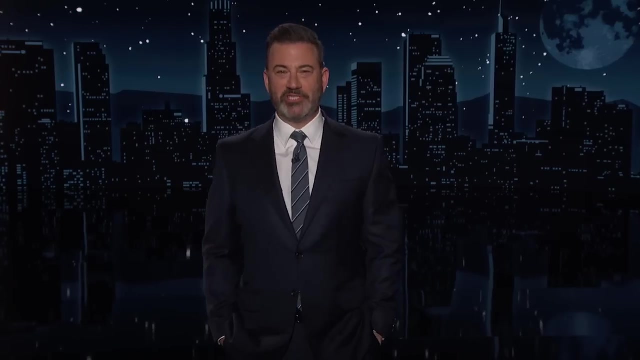 Trump handles an eclipse the same way he does a porn star: Unprotected. That's the kind of man he is. And then his team, his election team, used the eclipse to make some kind of a point on Truth Social. We will save America by plunging it into complete and total. 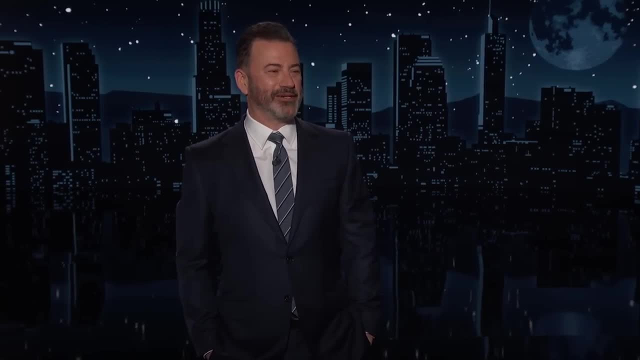 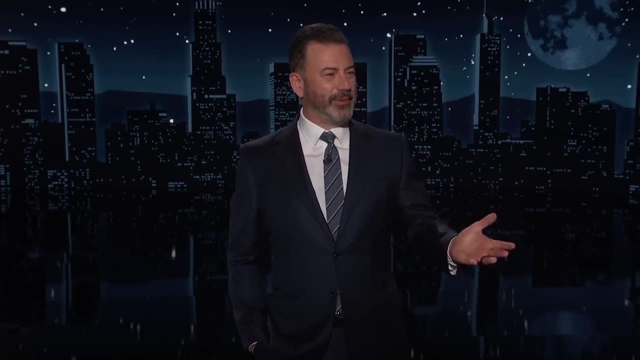 darkness with my giant head. Nothing says I won't be a dictator like blocking out the sun. You know Marjorie Taylor Greene. I feel like this didn't get enough attention. On Friday, I think, she tweeted about the earthquake in New York and the eclipse, saying God is sending America. 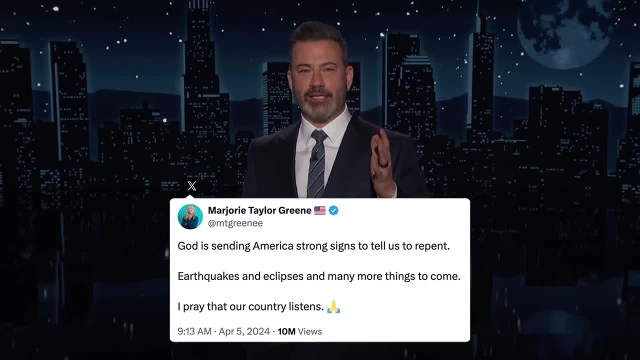 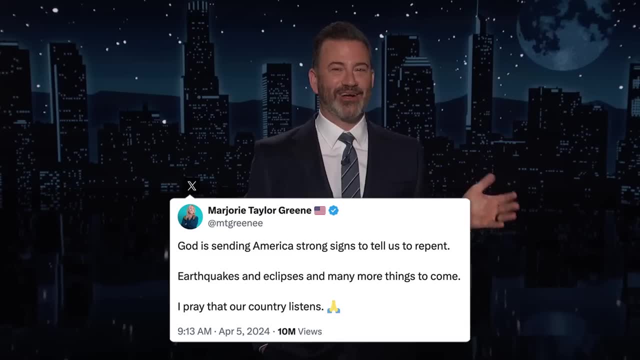 strong sun, Strong signs to tell us to repent. Earthquakes and eclipses and many more things to come. That's right. there's a Godzilla coming too. I don't know if you guys know that. I pray that our country listens. 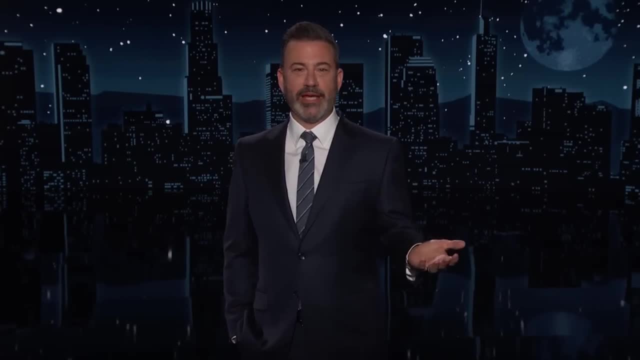 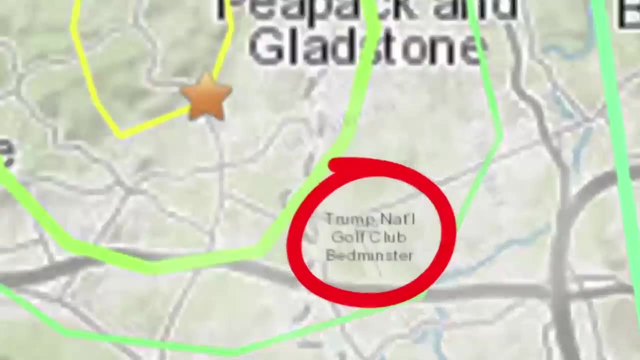 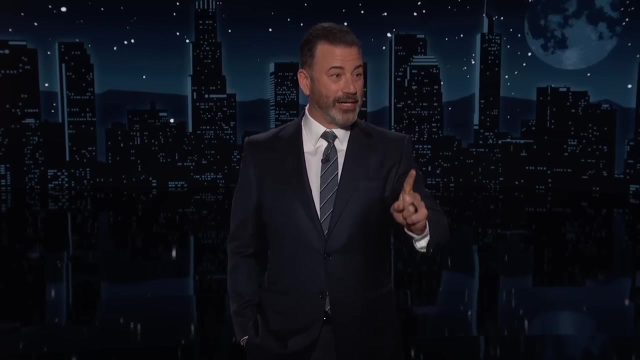 And what makes this spectacular display of dim bulbury interesting is that the epicenter of the earthquake in New Jersey that she thinks God made happen to warn us was literally on Donald Trump's golf course. That is not a joke. That's where it God put it, on the Tan Andreas. 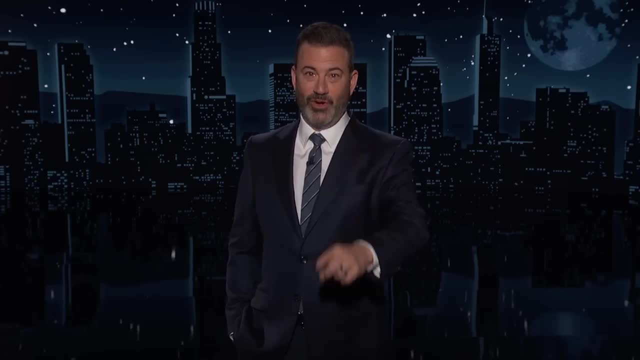 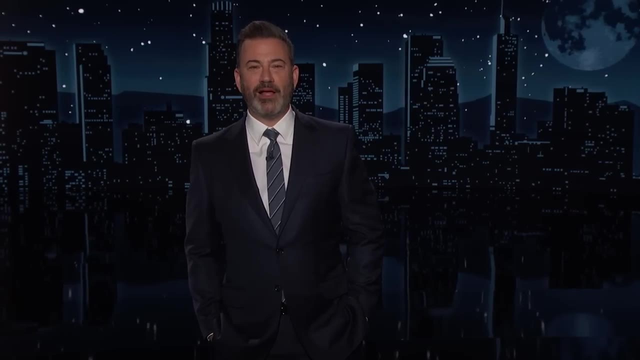 Fault. to warn us. to warn us. You know, at Mar-a-Lago- this is good- Trump accepted an award on behalf of his wife, Melania, who is apparently too busy not attending to attend. We want to take this opportunity. 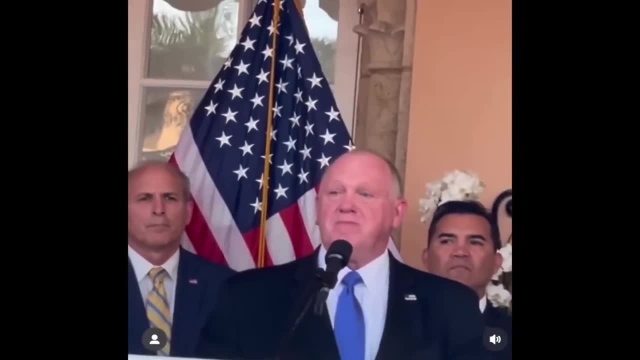 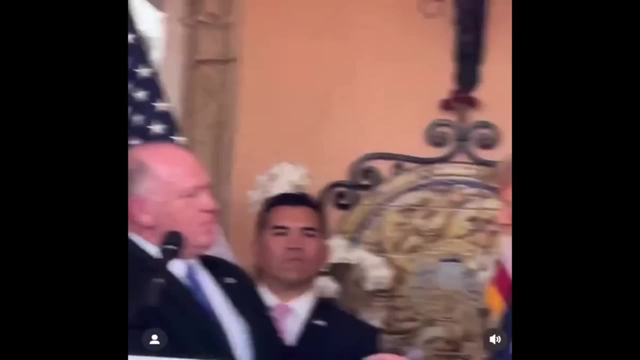 I know First Lady couldn't get here, but we want to give Melania Trump the Child Advocacy Award because she said she just she did so much for children when she was First Lady. So, sir, this is for Melania, Thank you. 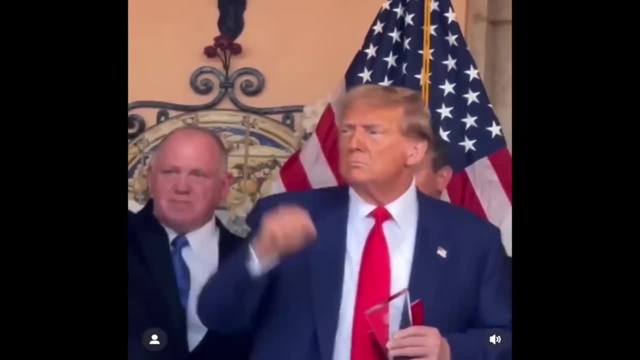 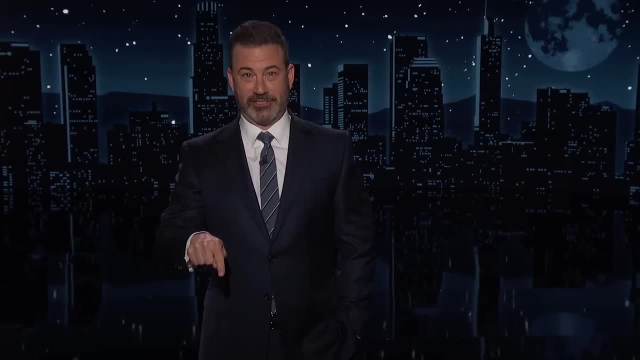 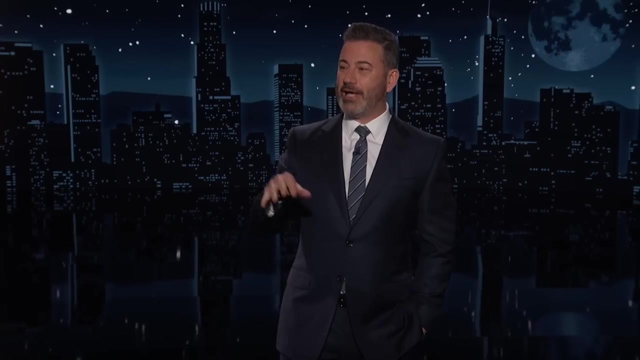 That's right. She couldn't be here to accept an award at her house. OK, She wanted to be here and she was, but she also wasn't. Melania was. that was the Child Advocacy Award and it was given to her by Trump's former director of ICE. 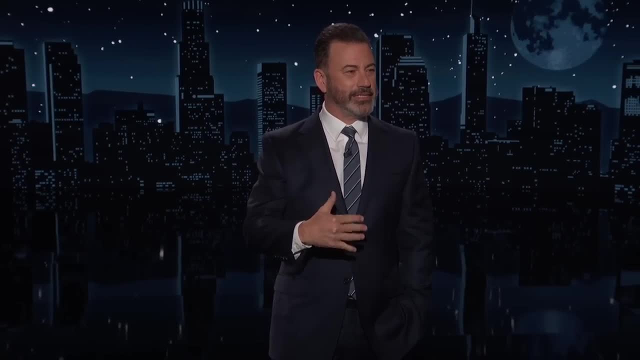 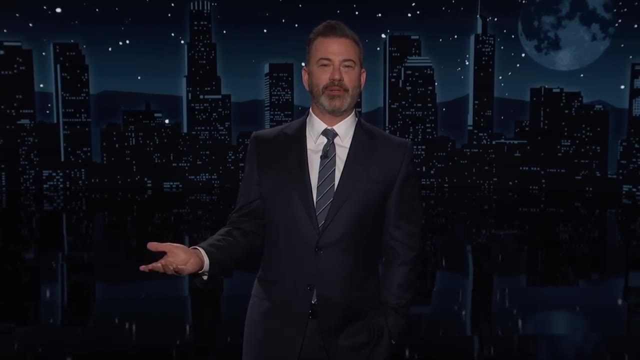 which is not unlike getting a Teen Choice Award from R Kelly. It doesn't really, and I don't know why this was necessary. Here's just a here's a tip If you're making up an award in the first place. 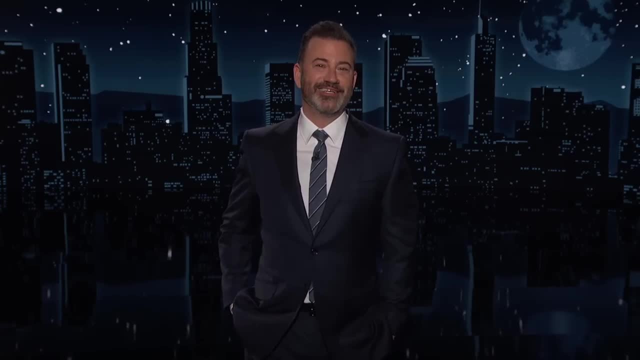 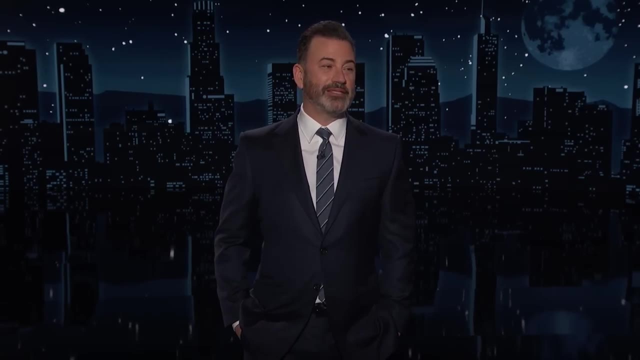 you can give it to the person whenever they can make it downstairs. You don't have to. Melania did make a rare appearance alongside her husband at a fundraiser on Saturday night. Trump claims he raked in $50 million Saturday night, which seems high, but he's not one to exaggerate. 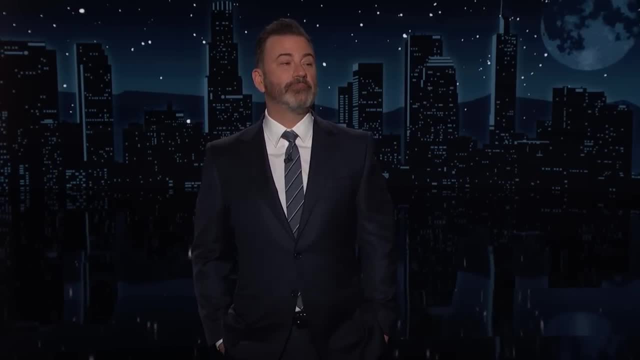 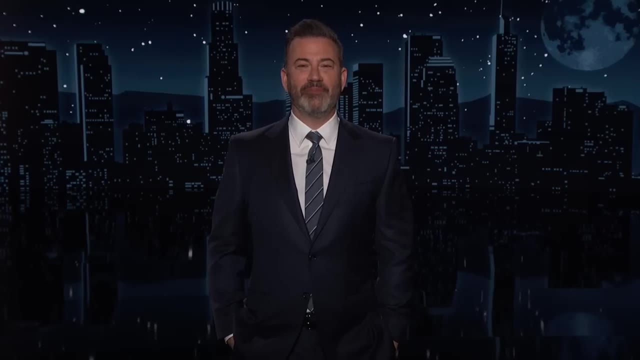 At the fundraiser. he said he wants immigrants to come from nice countries like Denmark and Switzerland and Norway. Whenever Trump says nice, he means white. But He's also working hard to reimagine his official stance on abortion. You know, secretly he's for it, he's very for it. 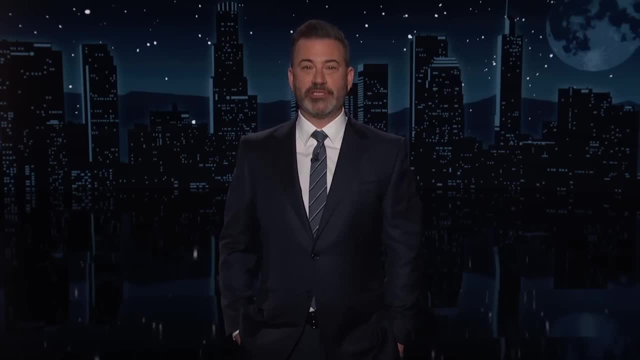 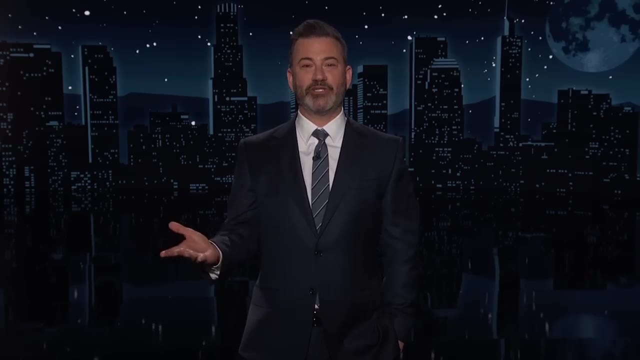 but he can't say that And, of course, after appointing enough Supreme Court justices to take away a woman's right to choose, a lot of Americans are upset, even Republicans. So, in an effort to have his cake, and eat it too. 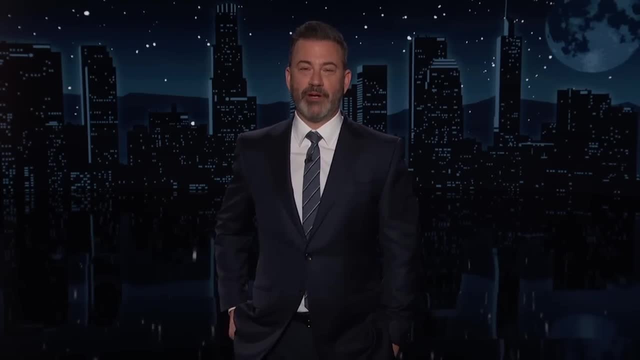 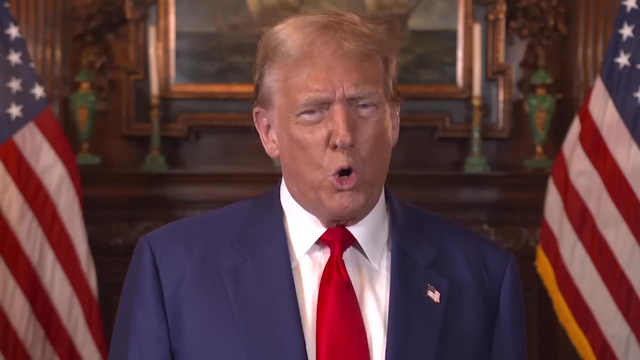 he got a hot new spray tan and he lined up in front of two enormous American flags. It must be remembered that the Democrats are the radical ones on this position because they support abortion up to and even beyond the 90s. The Democrats are not the ones to support abortion. until the end of the 19th month. The concept of having an abortion in the later months and even execution after birth- and that's exactly what it is: the baby is born, the baby is executed after birth- is unacceptable and almost everyone agrees with that. 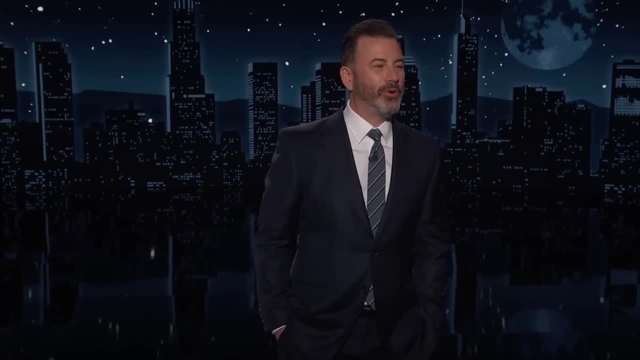 That's right. You didn't know. there were baby firing squads going on around here And to prove it, Trump is going to allow them to abort, Eric and Don Jr, At age 40.. Here's something Trump might want to look into. 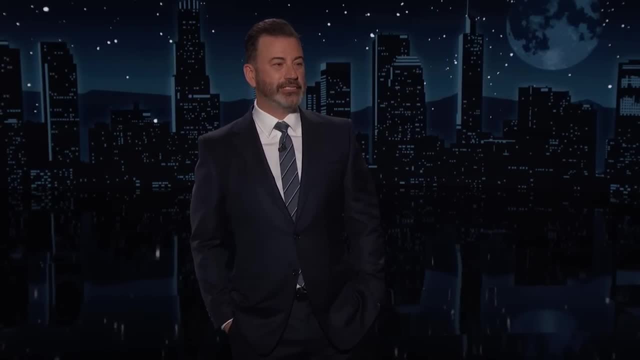 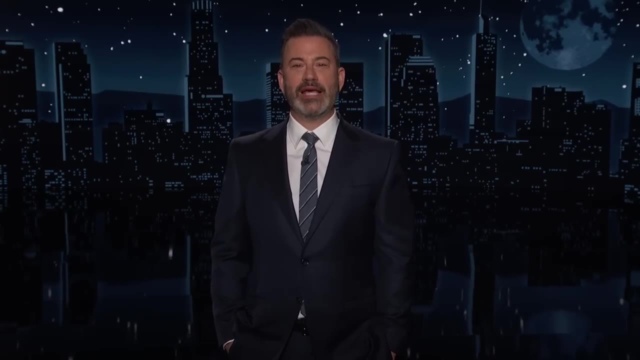 Of all the stuff artificial intelligence can supposedly do, this is one I know. I never imagined There's an app that uses AI to determine if you have an STI, which used to be called an STD until they changed it to confuse us. 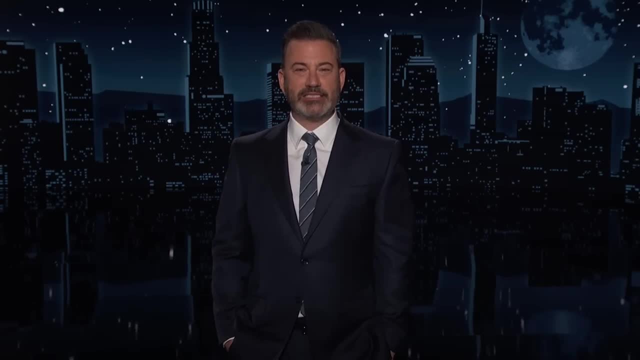 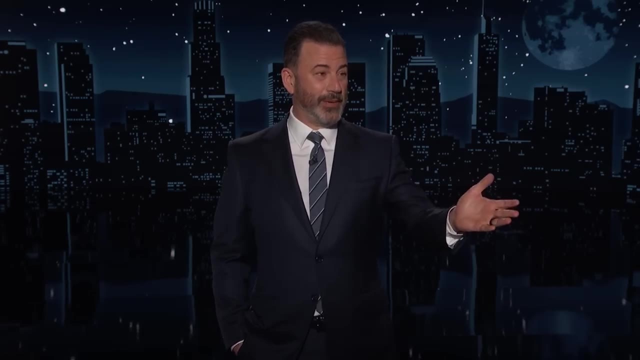 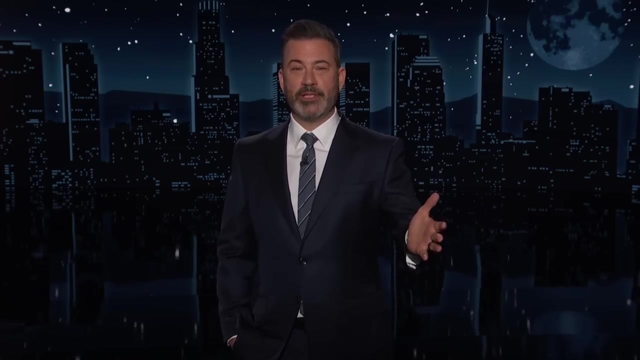 But UFO is now an UAP and STD is an STI. If you come in contact with either one of them, call the Space Force immediately. But somebody at this startup out of San Francisco launched an app called Kalmara, which is trained to recognize diseased human peni. 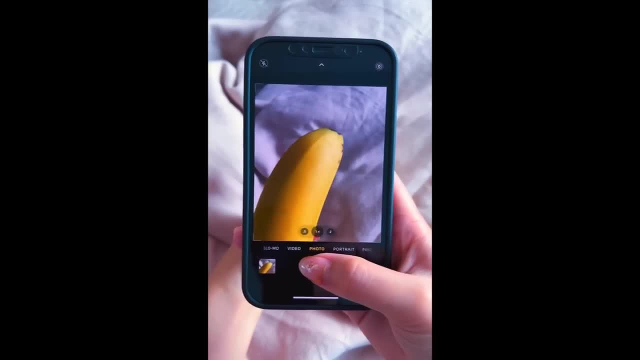 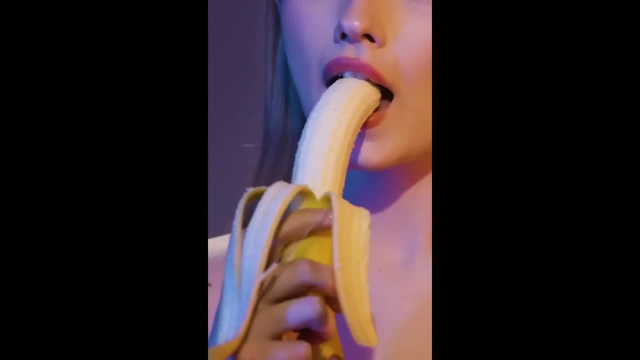 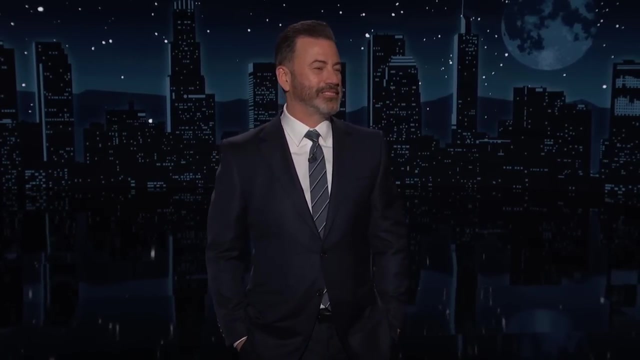 Right all night. right right all night, Feel, feel, feel. so right, Wait a minute, Dave, It's clean. you give it a bite and then you know It's an interesting idea. The only problem is doctors looked into it. They say it isn't effective. Kalmara claims It claims its accuracy rate is 65% to 95%, which an expert described as terrible. Oh, you're 65% herpes-free. Let's do this Back to this eclipse. 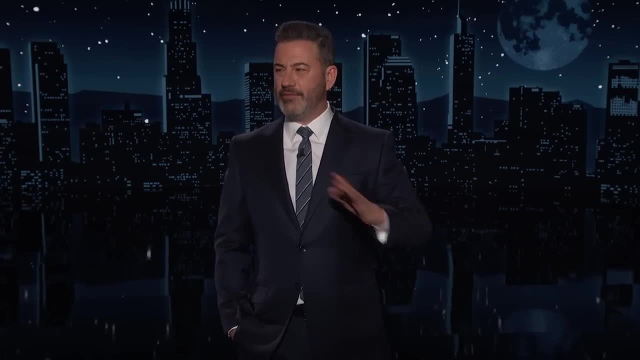 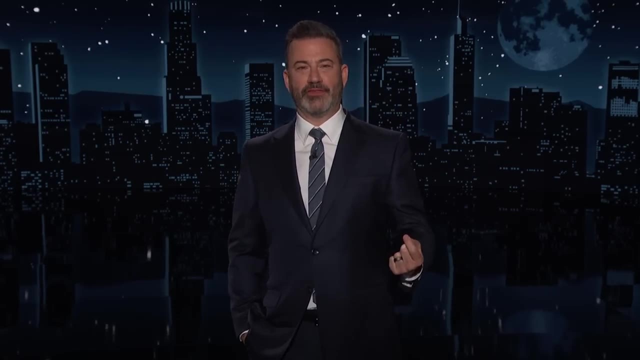 You might imagine, this was a very big deal for the Weather Channel, Even though I'm not sure it qualifies as weather. this reporter was on the scene in Texas today. She showed a tremendous amount of enthusiasm for the moon blotting out the sun. 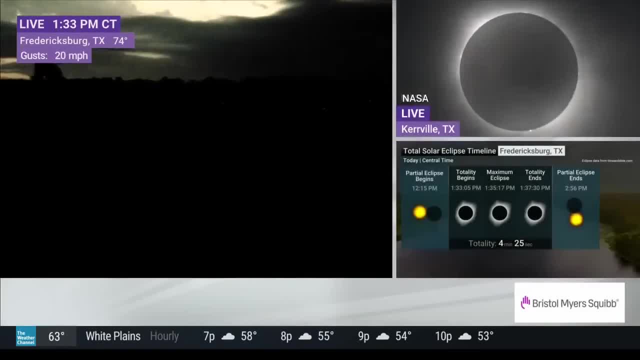 I can even see a blue spawn right there. Come on, Come on. Oh my God, Four minutes. The crowd is willing it. Yeah, Whoa, We can see it Just for a minute, Just for a second, But I'll take it. 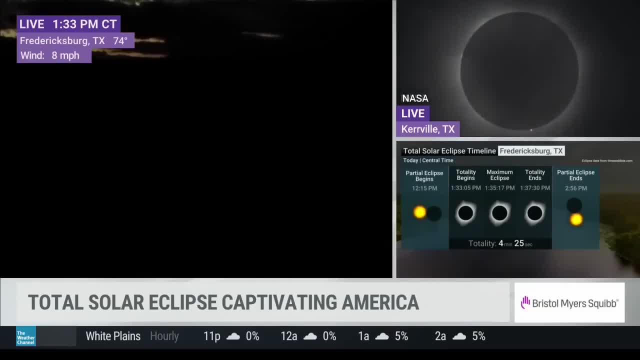 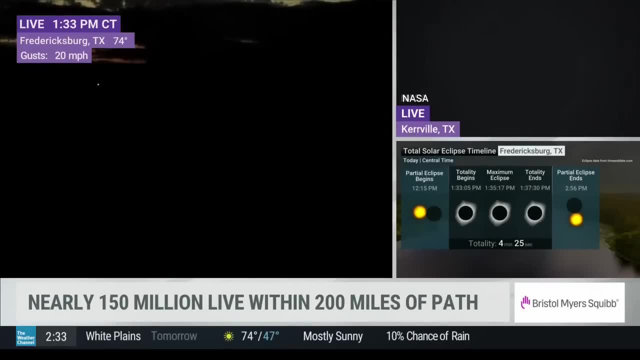 I will take it, Yuck it in. Oh my God, We got it. We got it. Oh my God, Lauren, look out, I'll have what the eclipse is having. That is, That's great, That's like. 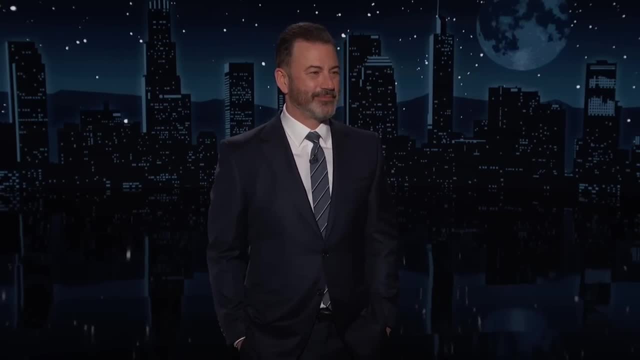 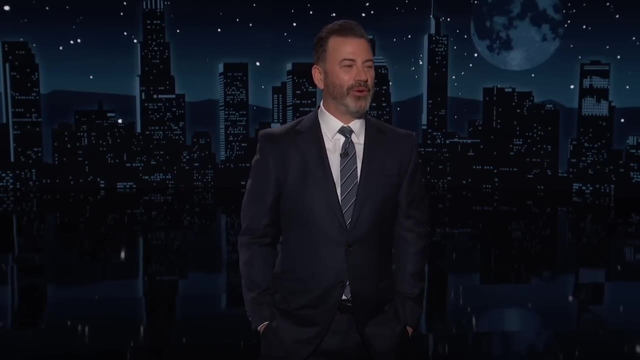 Sounded like Lauren Boebert Beetlejuice. That was wild. It's exciting, I guess. When I came into work this morning, everybody was in the parking lot looking at it, which made me wonder how many people know what an eclipse even is. 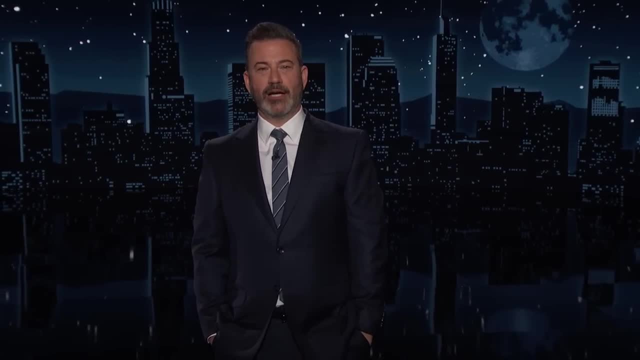 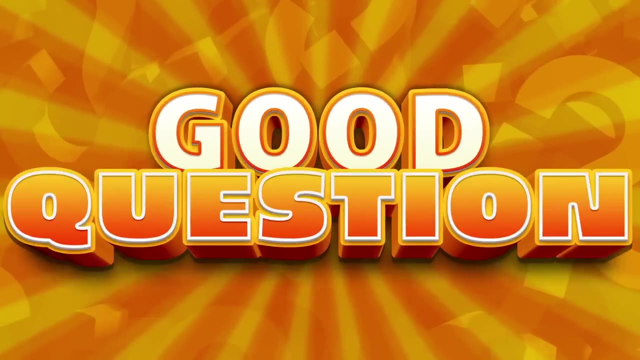 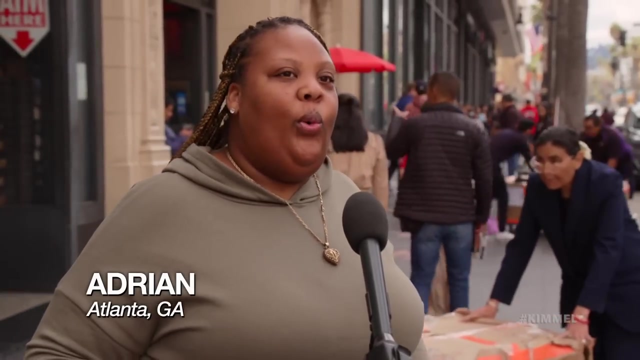 So we went out on Hollywood Boulevard. We asked pedestrians a simple question, a good question even. We asked: what is an eclipse? And here's what it is: What is an eclipse? What is an eclipse? Ooh, I don't know what it is. 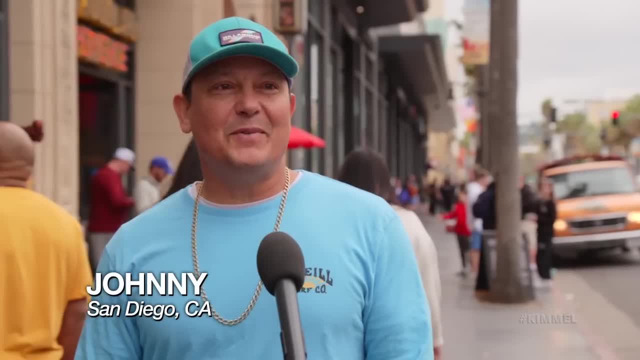 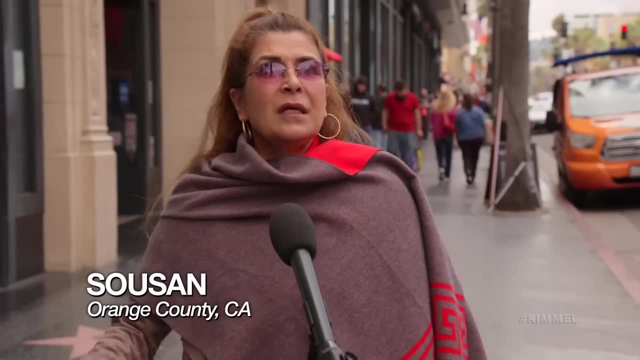 I know we've got to wear sunglasses for it. I don't know. An eclipse in a movie. What is that? I don't know. This is a trick question. It's the When the moon is under covered by the clouds, I believe. 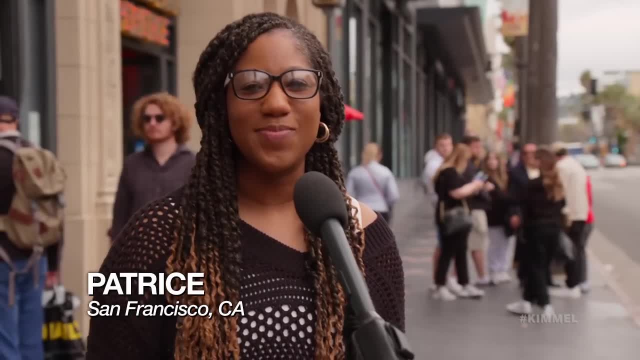 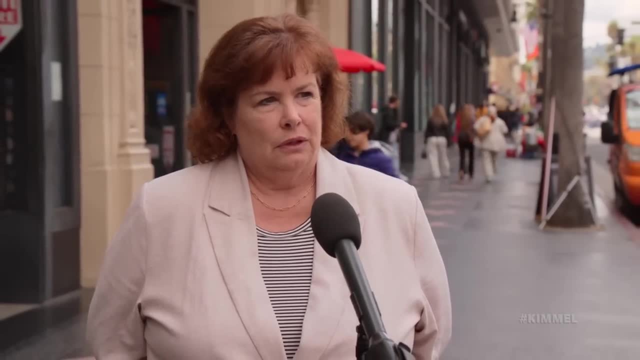 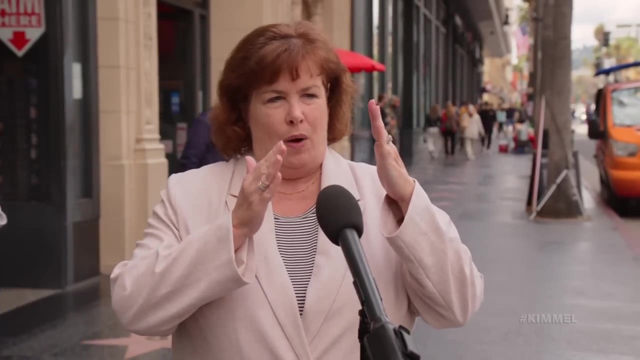 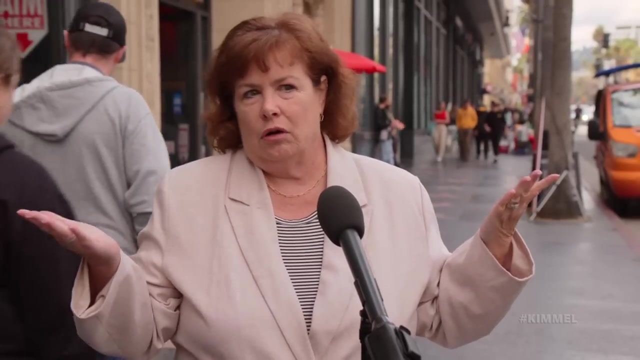 I believe it's like when the moon and the sun collide and there's a space in between. What happens during an eclipse? It is when It It has to do with the sun, in that it is when the sun becomes covered and it ends up being dark for a while. 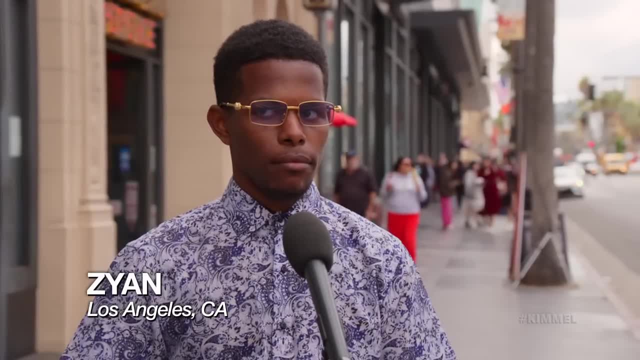 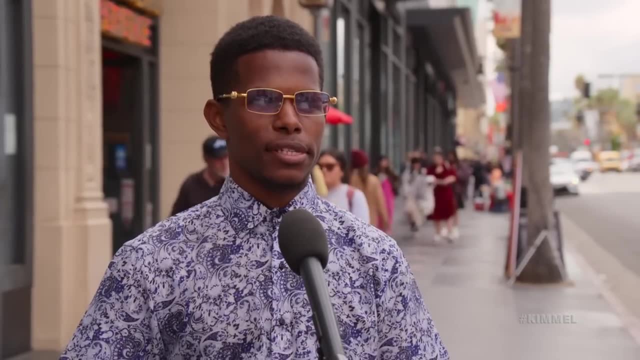 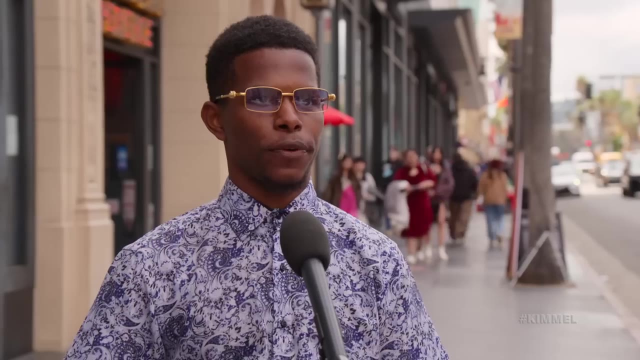 How long do you think the eclipse will last? I think 72 hours, three days, Because the reason I think that the solar eclipse may happen for three days is because that's what Gilbert told me Gilbert was referring. He was referring to the three days. 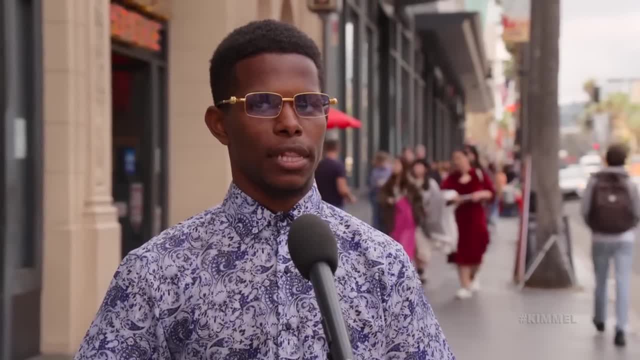 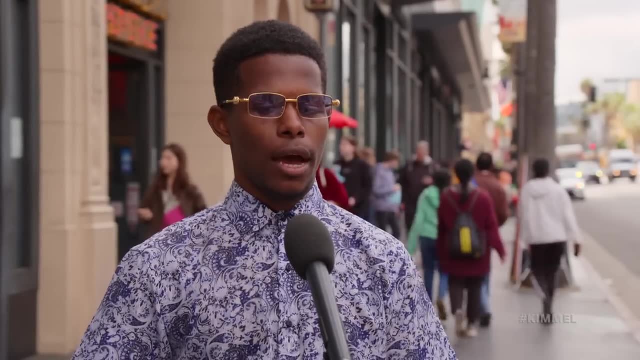 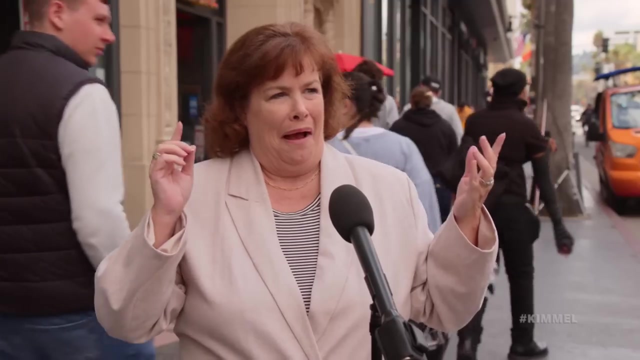 that people are going to have to stay inside. There's going to be a lot of crime happening, There's going to be a lot of dangerous activities, more than what we already experienced. What does it become covered with? I, I think with another planet or 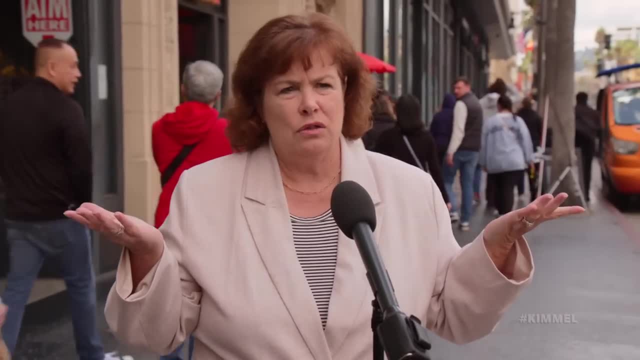 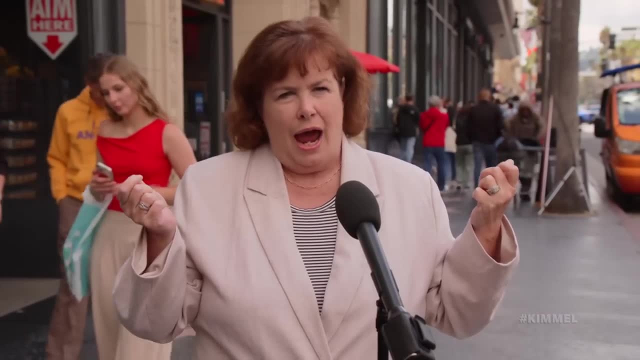 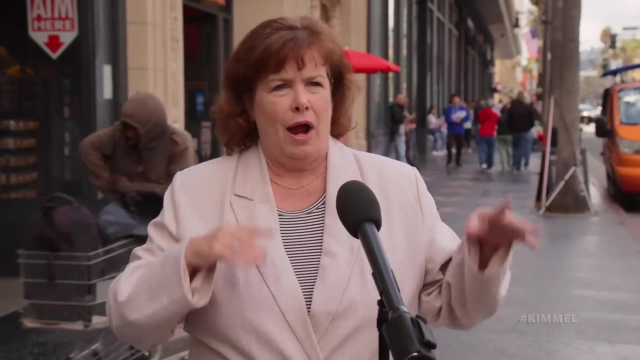 Yeah, Yeah, because it wouldn't be clouds. Do you know a planet? Was it Pluto? I don't remember, and I don't know where this one is, but I think it's happening in Mexico, Because we were on a plane. 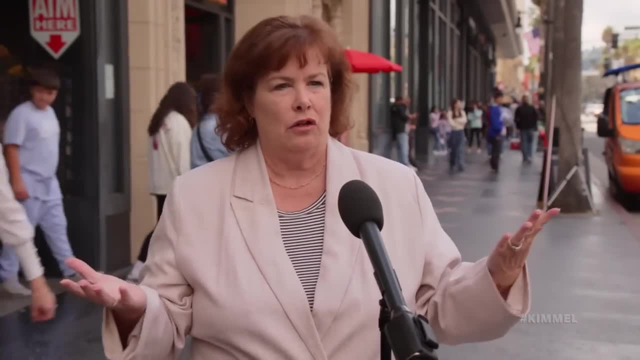 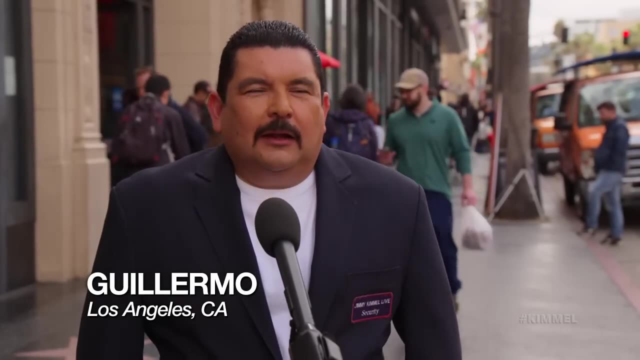 and people were all going on a cruise to Mexico to see the eclipse. So I think that's where you see it. What is an eclipse? An eclipse, Oh, an eclipse is a thing that is in the air. It doesn't.